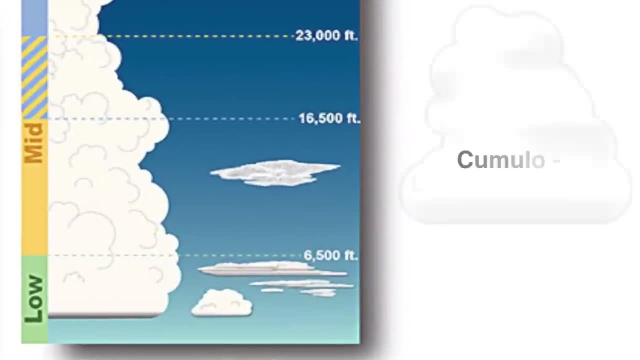 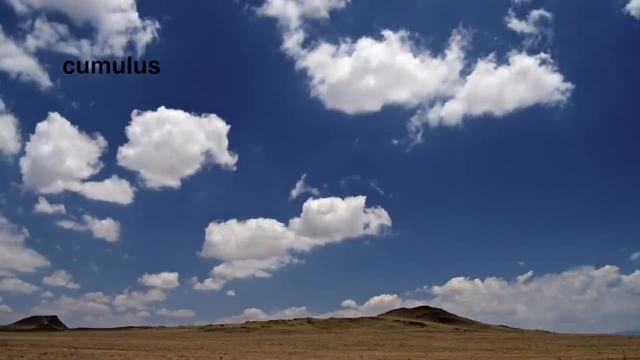 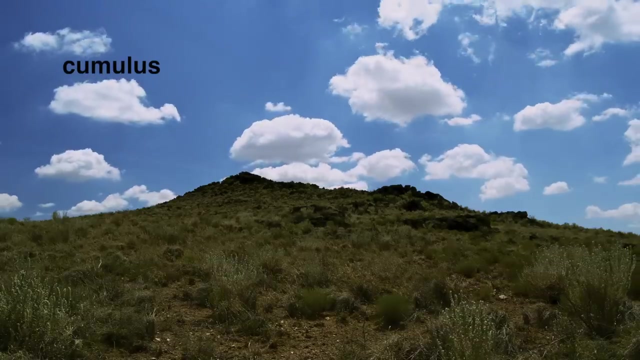 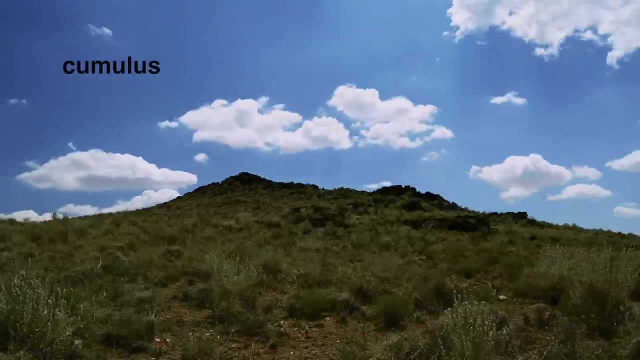 more recognizable cloud types. cumulo is latin for heap or pile, and cumulus clouds can often look detached or isolated from other clouds, and they'll often appear as fluffy white cotton balls or perhaps even cauliflower. these clouds are considered low-level clouds, usually forming between a few hundred to a few thousand feet above the earth's surface in the desert southwest and 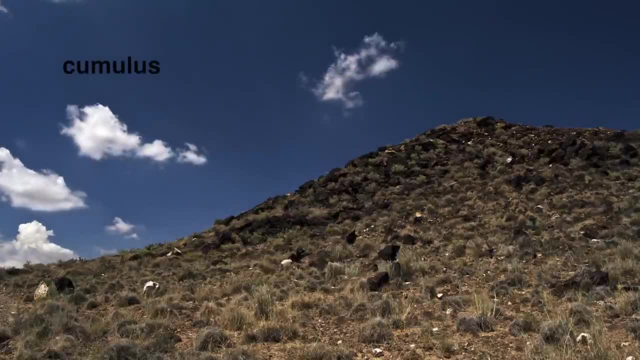 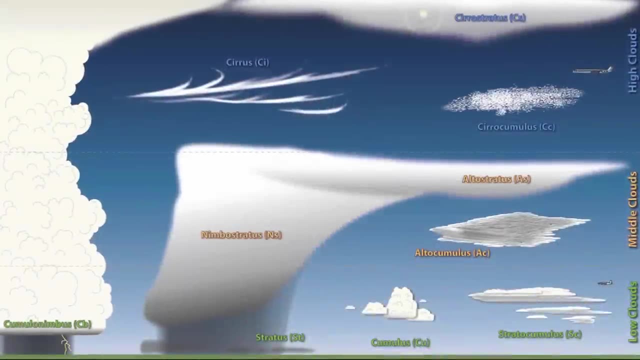 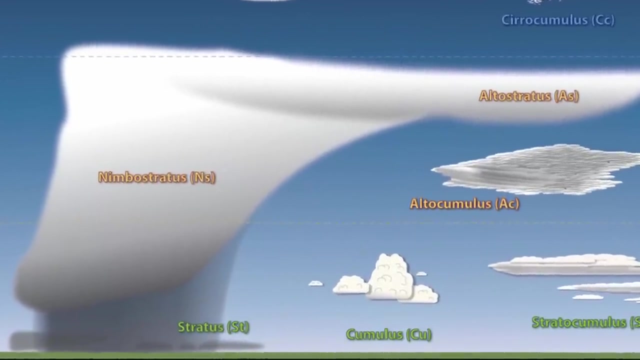 much of new mexico. these cloud bases will often form at even higher levels than other parts of the country due to the warm and arid conditions within the southwest. stratiform clouds or Clouds often appear as a sheet or layer of cloud that exhibits little definition or features. In other words, they will typically appear as a hazy, white or gray. 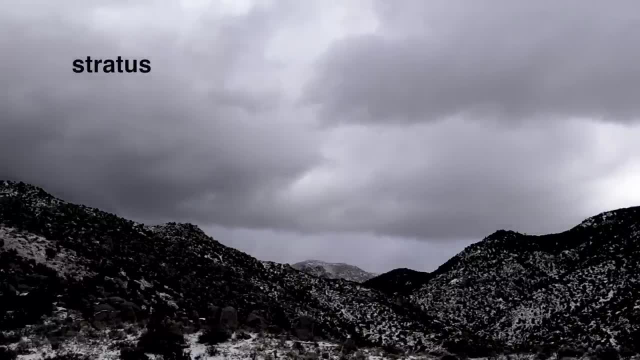 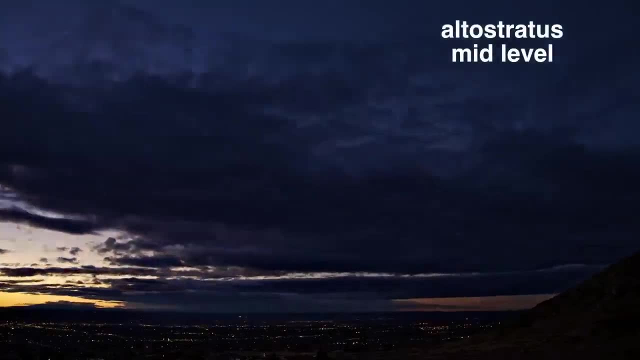 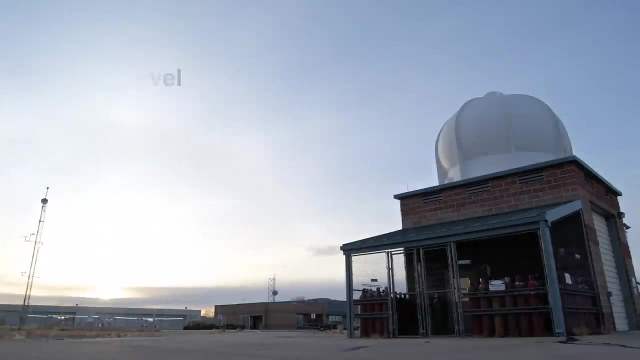 mass Stratus clouds are primarily thought of as low clouds, but they can also be observed in the middle to upper parts of the atmosphere as well. Mid-level stratus clouds are referred to as altostratus, and high-level stratus clouds are commonly identified as cirrostratus. Nimbo-form clouds are also. 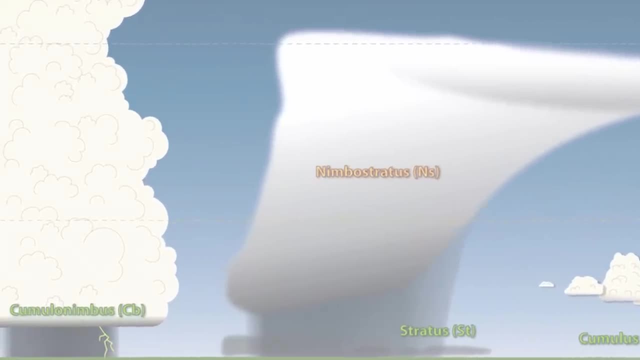 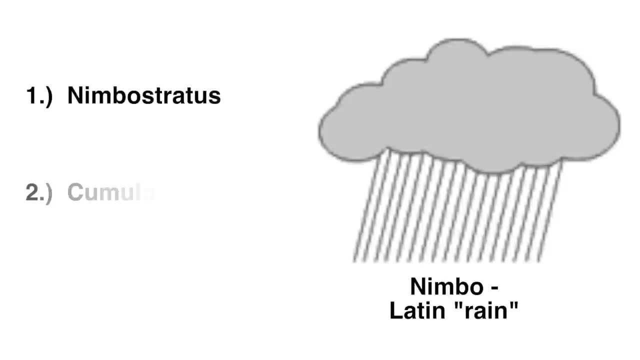 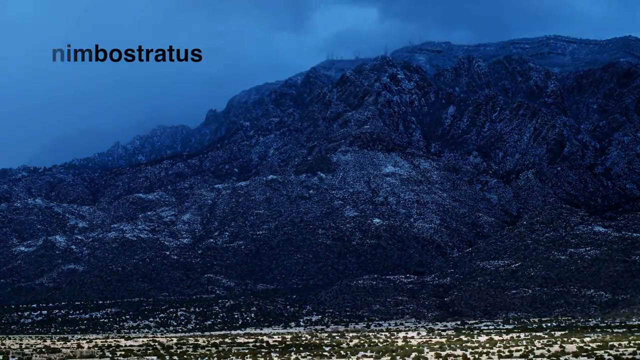 representative of a hybrid or combination of different cloud categories. Nimbo is Latin for rain. The two common nimbo-form cloud types are nimbostratus and cumulonimbus. As you can probably guess, nimbostratus are layered clouds producing rain or precipitation. These clouds can extend. 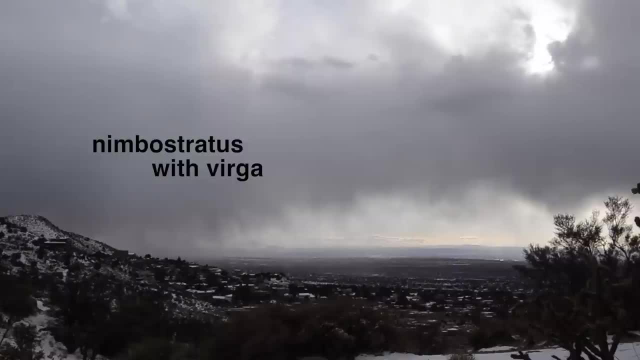 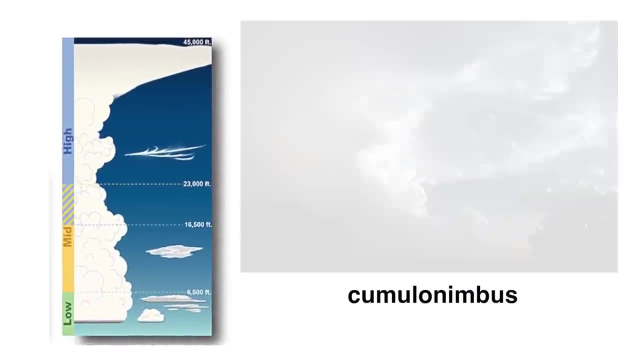 into the middle to upper parts of the atmosphere, But they are typically only seen in the lower parts, since they will usually obscure any. clouds above Cumulonimbus are also a unique hybrid of cloud that extends from the lower to the upper parts of the troposphere and are 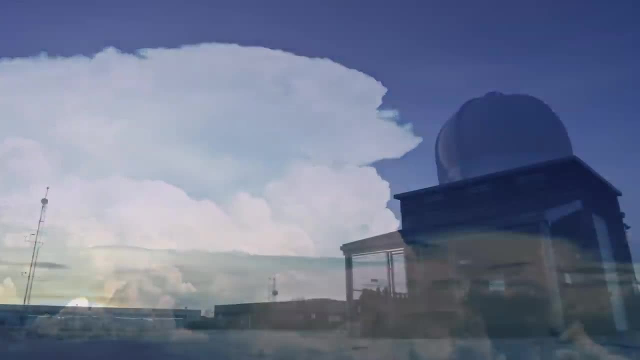 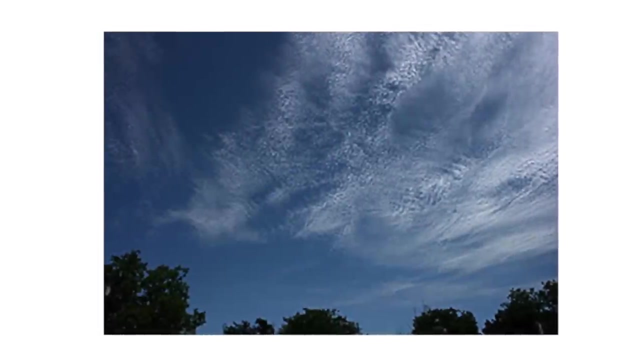 otherwise known as thunderstorm clouds. We briefly mentioned cirrostratus, but another high-level cloud is cirrocumulus. These are similar to altocumulus, the difference being that altocumulus is a cloud that extends from the lower to the upper parts of the troposphere. 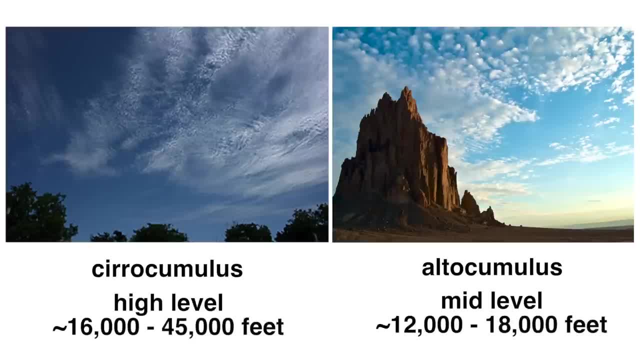 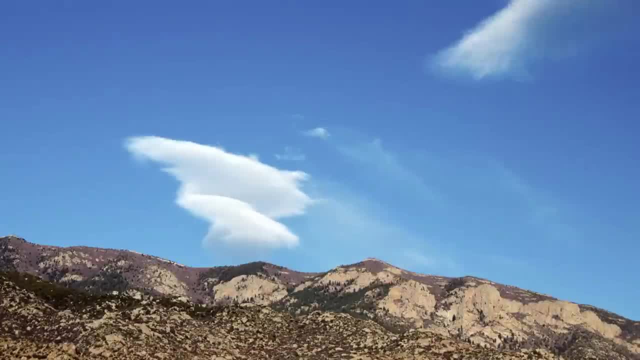 The altocumulus forms in the mid-levels of the troposphere, while cirrocumulus clouds are in the highest part of the troposphere. Altocumulus clouds have some variations of their own. One such variation that frequents New Mexico is the altocumulus standing lenticular, sometimes simply.